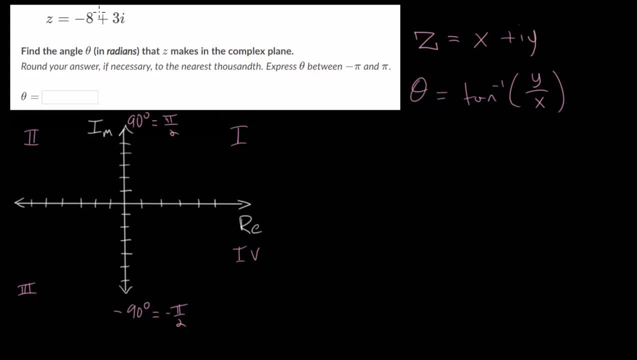 more careful with this formula. So let's start by first plotting this complex number. And it has a real part of minus 8, and we will use a scale of 2 for the x values. So that's the real part of minus 8, and we will use a scale of 2 for the x values. 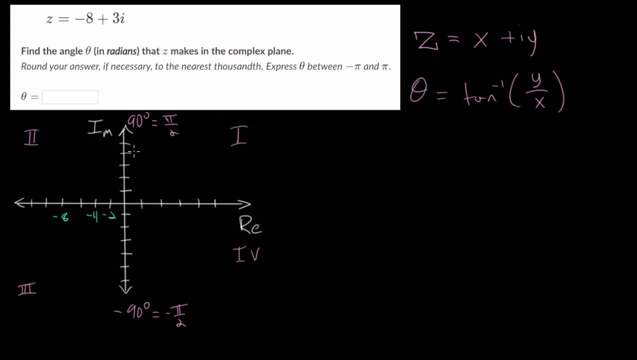 So that's the real part of minus 8, and we will use a scale of 2 for the x values. this right here will be minus 8, and for the y values we can use a normal scale of 1, so this will be at 3i. so our complex number is right here and we can draw a line connecting that. 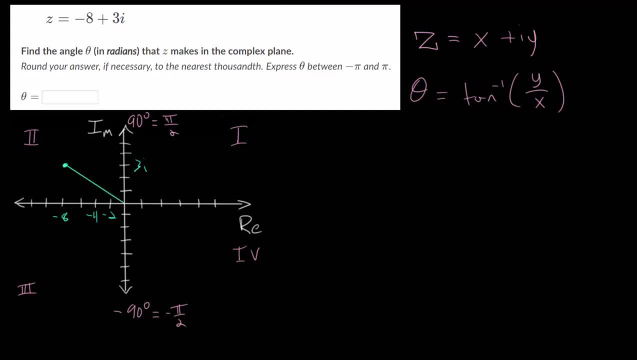 complex number to the origin, essentially creating the vector for this complex number. if we want, we can draw in the arrowhead and remember this vector has a length, a magnitude, also known as the modulus of the complex number. but for this particular problem we're not concerned with 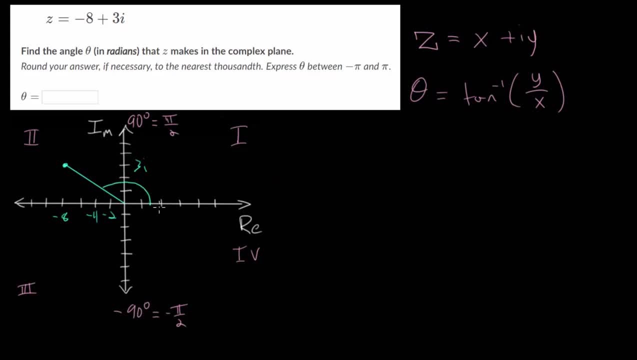 finding that what we need to find is the angle measured from the positive real axes, and we can call this angle theta, and we will need to measure it in radians. now, to find this angle theta, we can apply this formula and then we just need to be a little bit careful. so let's plug in the imaginary. 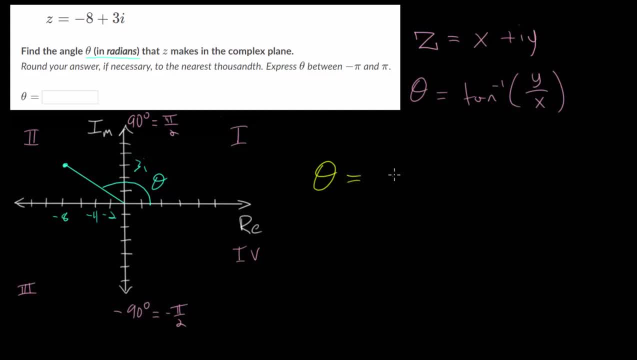 part of the complex number and we can draw a line connecting that complex number to the origin part and the real part. you have that theta is equal to the inverse tangent of the imaginary part, which is 3, divided by the real part, which is minus 8. and I should mention that this angle 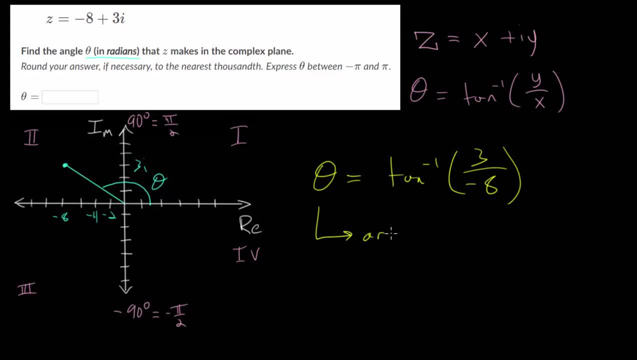 for complex numbers is often called the argument, so you might see this written as the argument of the complex number Z, and at this point we just need to plug in the real part of the complex number into our calculator. and we need to be careful, since we want the answer in radians, so make sure. 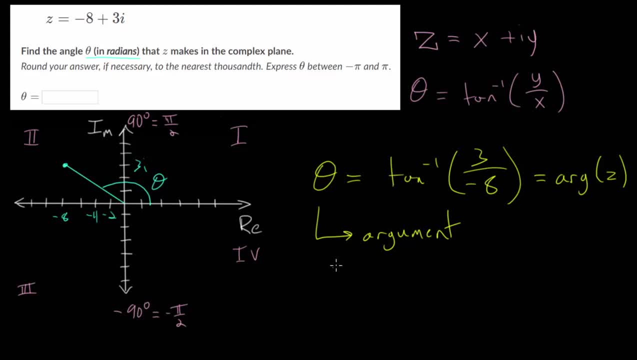 that your calculator is in radian mode and when we plug this in we get that theta is approximately. we'll have to round to the nearest thousandth minus 0.3587, which means we'll round this to minus 0.359. now you might notice the issue right away. this: angle is going to be 0.359 and we're going to have to round this to 0.359 and we're going to have to round this to 0.359 and we're going to have to round this to 0.359 and we're going to have to. 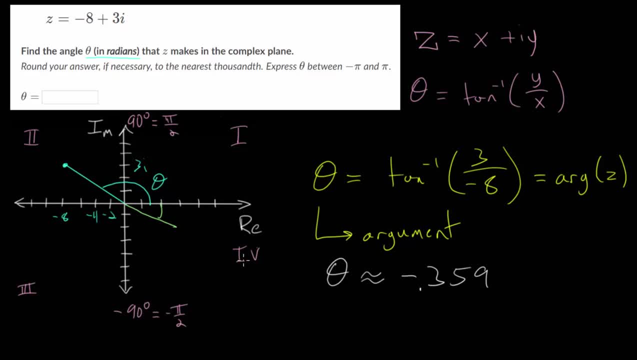 angle is essentially below the real axis and we know that our angle is measuring in the positive direction and it should be bigger than Pi, over 2 or 90 degrees. we want this in degrees. it's about negative 20, but the way to figure out what our angle is is to add 180 degrees. 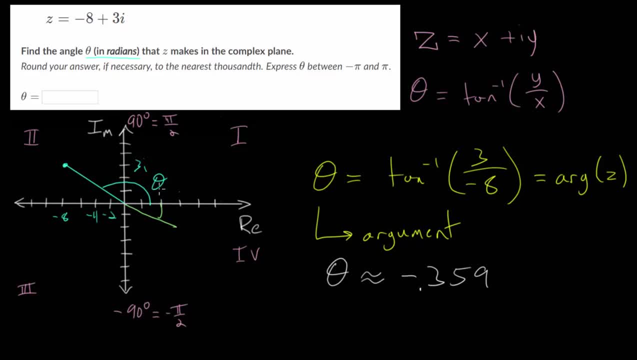 now, the way to remember- remember whether or not we are adding or subtracting 180- is by looking at the formulas for the tangent function. We can say that the tangent of the angle is equal to the tangent of pi plus the angle which is the one that we are using, or this is equal to the tangent of minus. 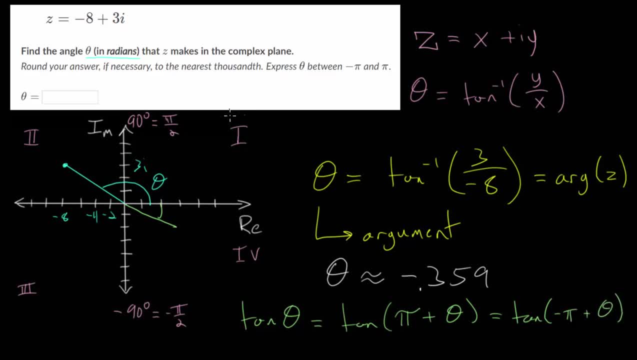 pi plus our angle, And if we are in the first or the fourth quadrants, we just use the normal tangent function. But if we are in quadrants two or three, we need to be more careful and use one of these identity functions And to determine which one to use we need to plot our point. 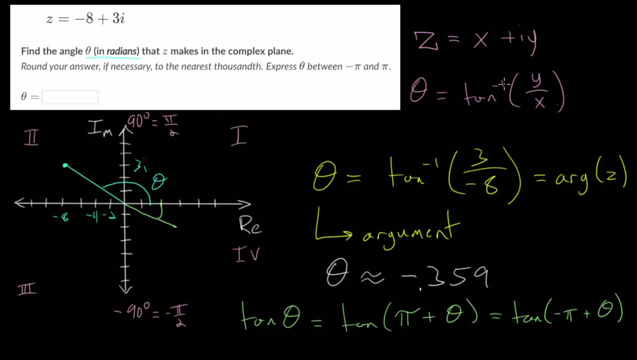 and consider what angle the formula gives us And by drawing in this angle, which is down here, we can recognize that we need to add to that angle, specifically 180 degrees or pi radians, To be able to get the angle we want. However, if we were in quadrant three and had some point, 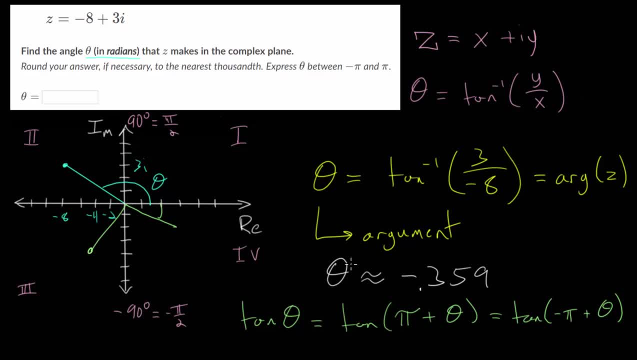 let's say down here, when we use this formula, we would plug in two negative numbers. they would cancel each other and we would get a positive value which would output an angle up in the first quadrant. But by using the geometry, by understanding where our point is and that its 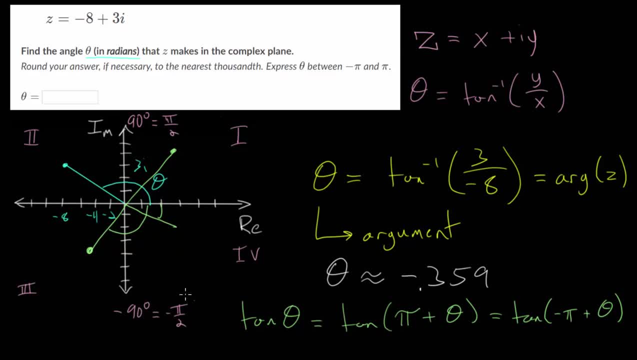 angle should be negative and more negative than minus pi. Then we can recognize that we have to take our positive Agora two. Then we can recognize that make us take our positive angle and subtract pi radians or 180 degrees to get the angle that we're actually looking for.